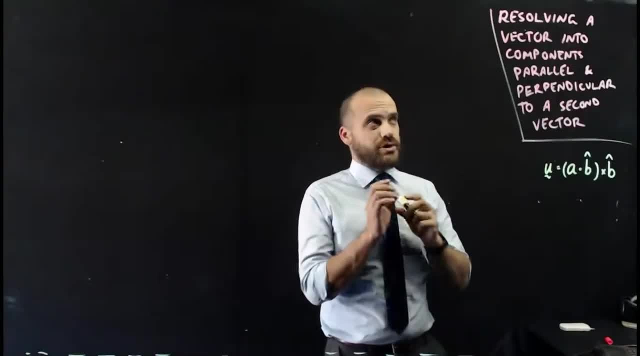 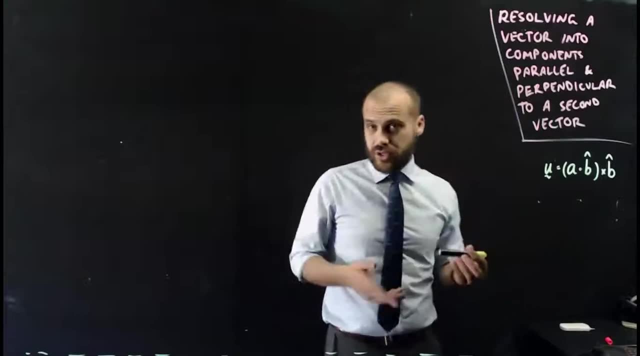 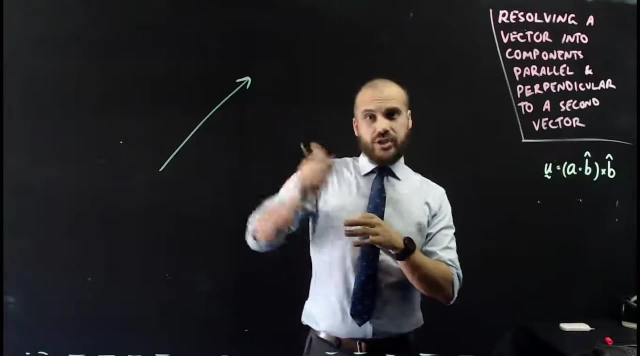 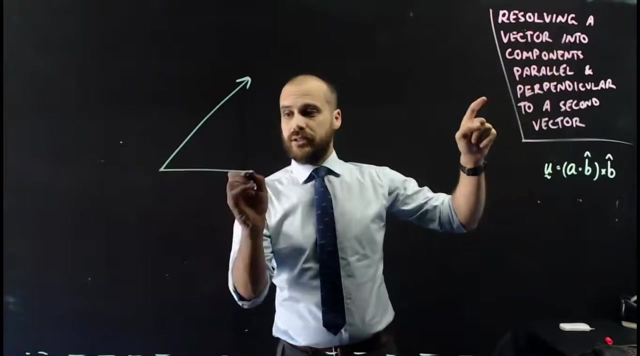 So usually I try to have short titles. This isn't one Resolving a vector into components parallel and perpendicular to a second vector. Now, we actually do this all the time. For instance, if I give you this vector here, we can talk about that in terms of an i and a j vector. What I'm doing is resolving a vector into components parallel and perpendicular to another vector. 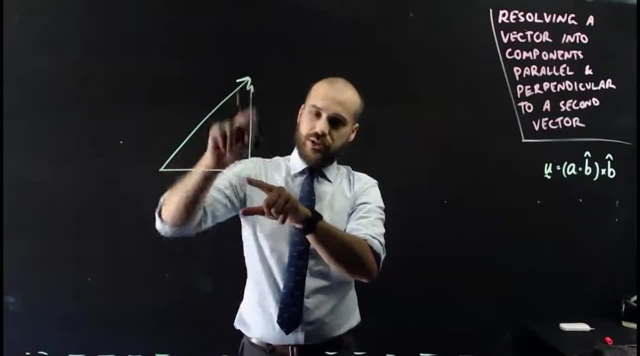 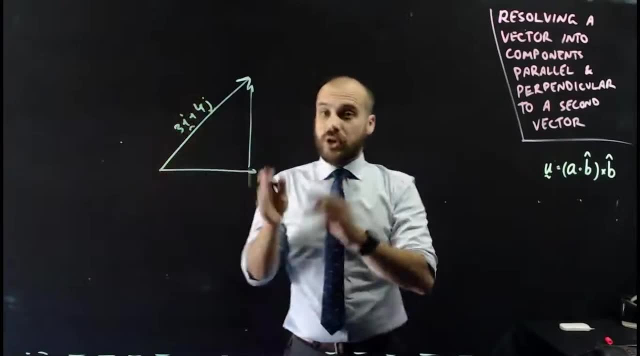 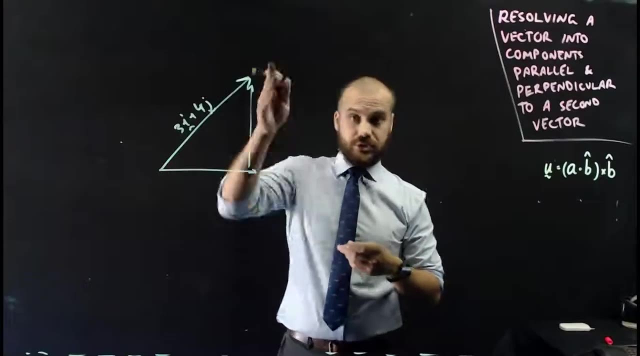 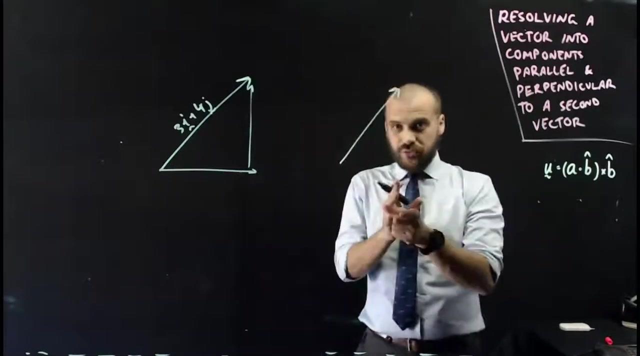 So I can call this vector 3i plus 4j. I'm resolving it into a second vector, something parallel to i and something perpendicular to i, which is j. Now, what we can do instead of that is take that vector and resolve it into components based upon a different vector. 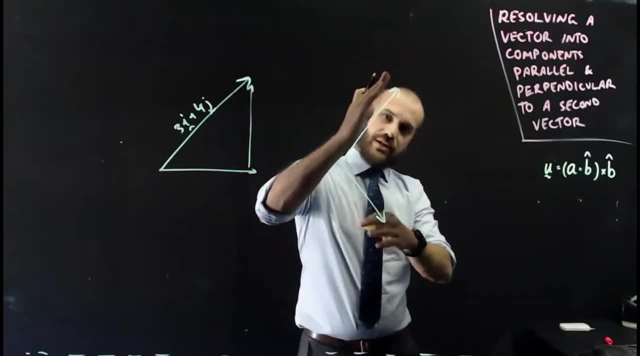 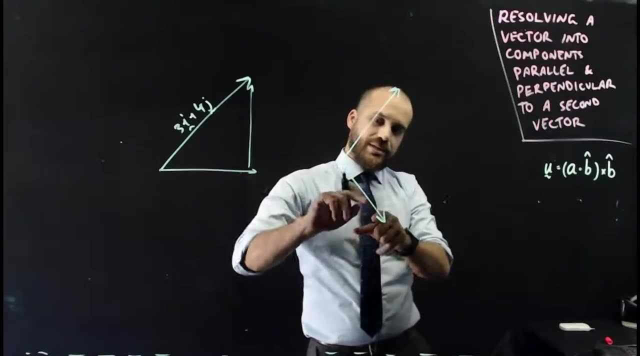 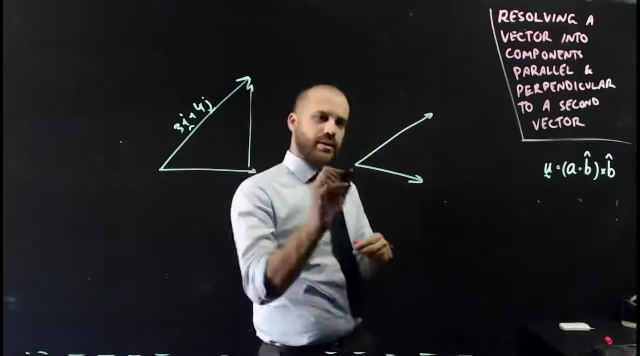 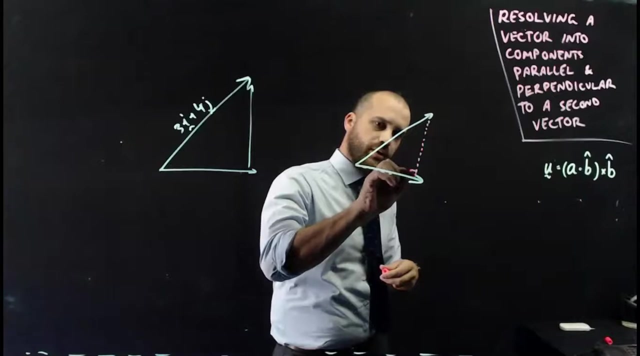 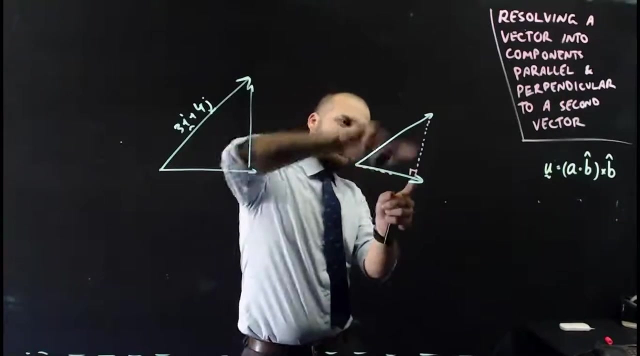 Now, in this case, I can take this vector and I can say: okay, how many steps in this component and how many steps in a component that's perpendicular to that. It wasn't a very good example, so let's use this one instead. How many steps along here and how many steps along here. We're no longer using i and j, We're using this as our i vector and we're kind of using this as our i vector. 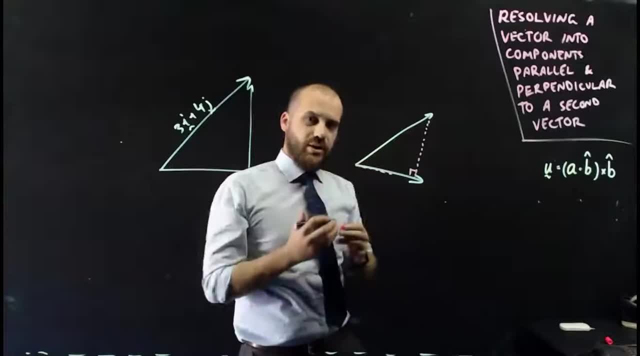 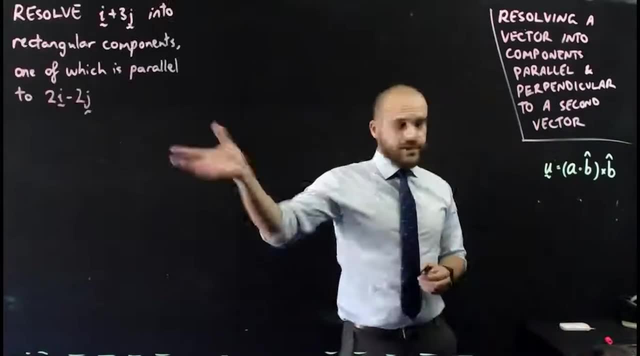 We're now using the perpendicular as our new j vector. Alright, so we're going to resolve a vector into components parallel and perpendicular to the second vector. I think it'll make more sense when we actually get stuck into it. Here's the sort of question we're going to answer. 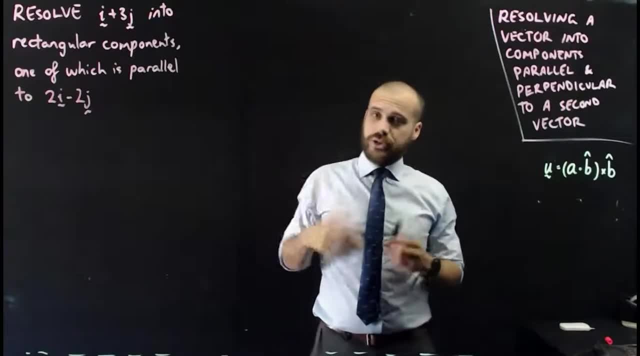 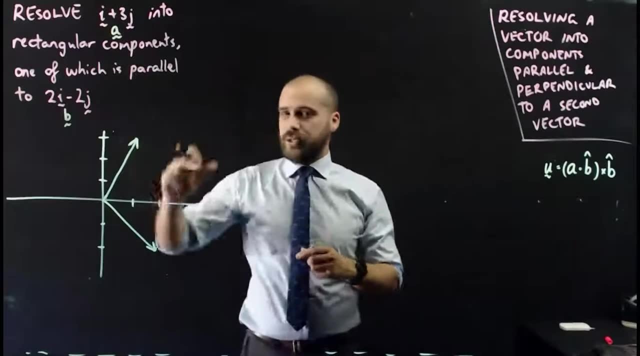 Resolve i plus 3j into rectangular components, one of which is parallel to 2i minus 2j. Let's draw a picture, Alright, so there's our two vectors. I'll call i plus 3j, a, so that's vector a there. 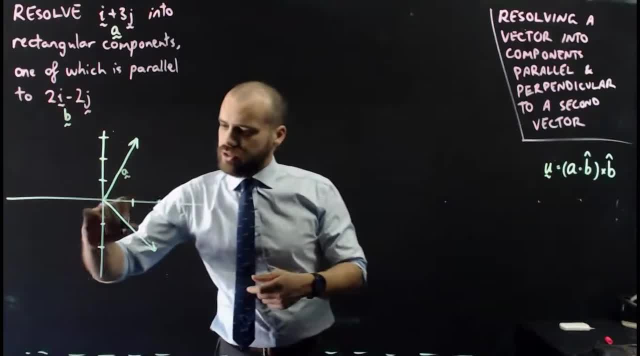 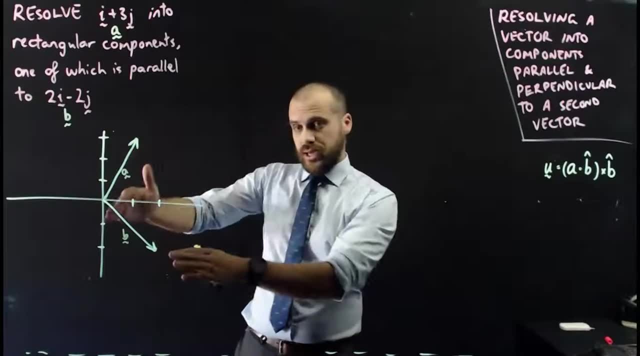 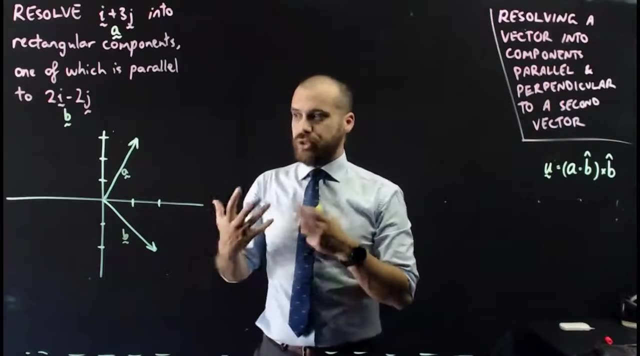 And this one is 2i minus 2j, so that's vector a. Now we need to be able to describe a- the vector a- in terms of b and another vector that's perpendicular to it. We're going to use a vector projection here, so let's project a onto b. 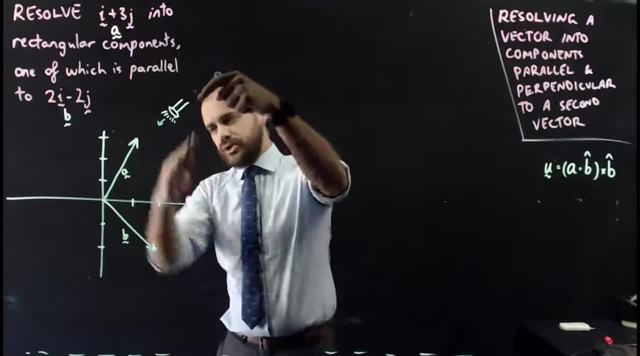 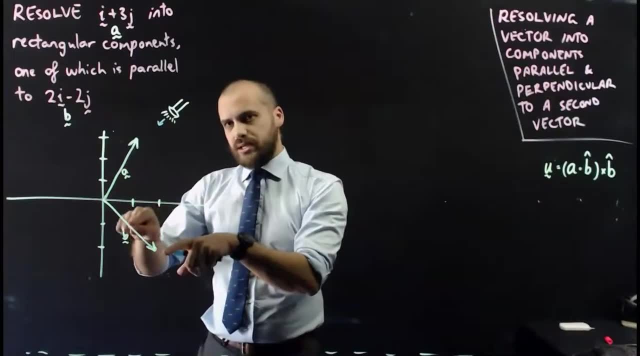 Now you can see that when I project- here's my torch- that's perpendicular to b. Remember that's how we do a vector projection. You can see that when I do that, I'm not actually going to cast a shadow onto b itself. 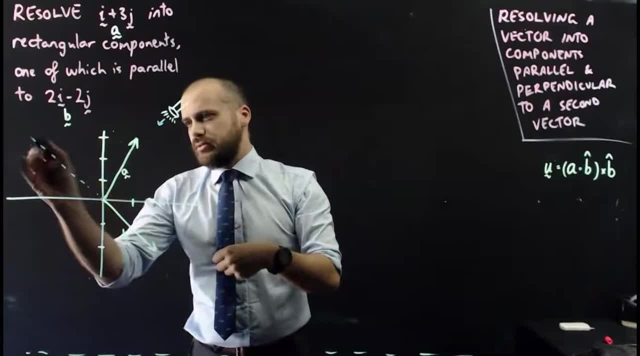 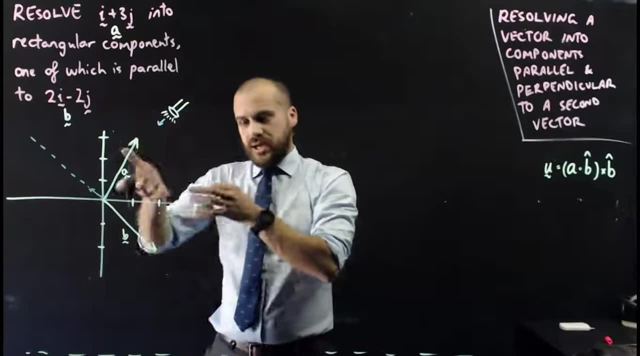 but I am going to cast a shadow onto b's expression, So I can just apply a shadow to b's expression. That's fine. That just means the shadow is like here And then the vector has a direction that's opposite. The thing that I'm projecting has a vector that's opposite there. 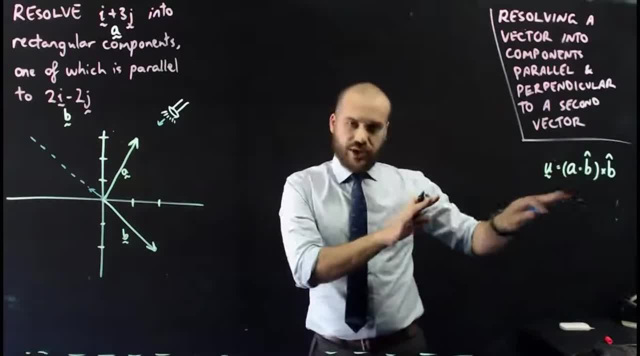 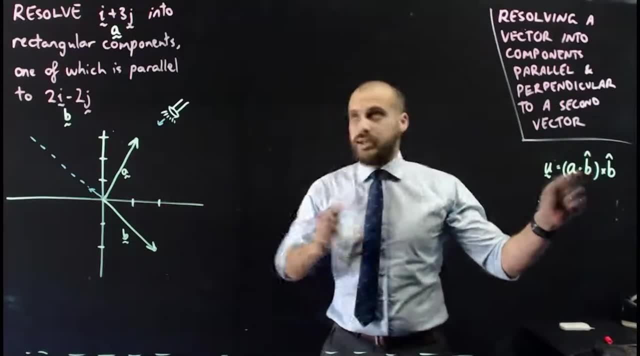 Alright, not that it matters too much. We can use our vector projection formula to come up with what our vector projection is, And to do that I'm going to need this guy here, my unit vector. So that's going to be the vector b. 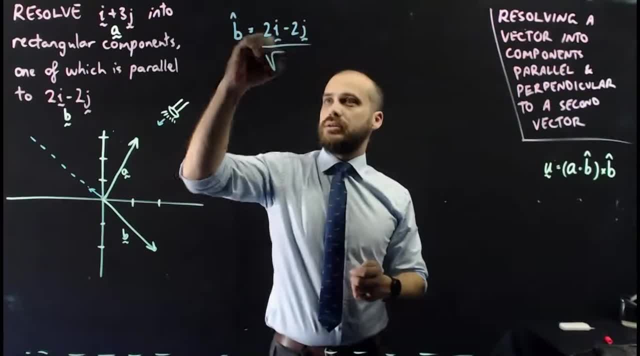 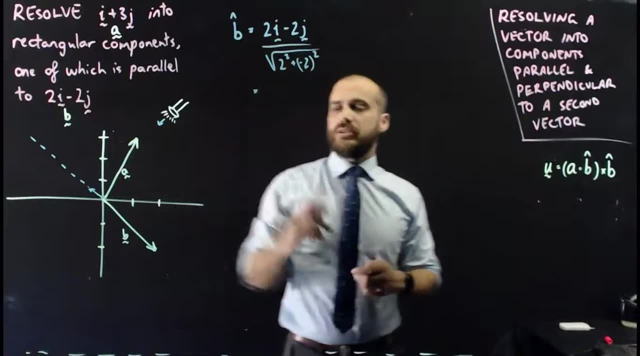 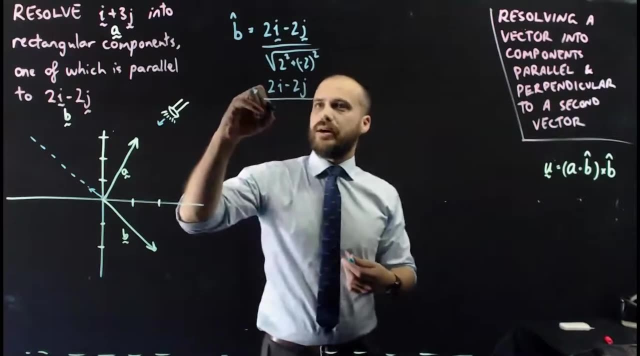 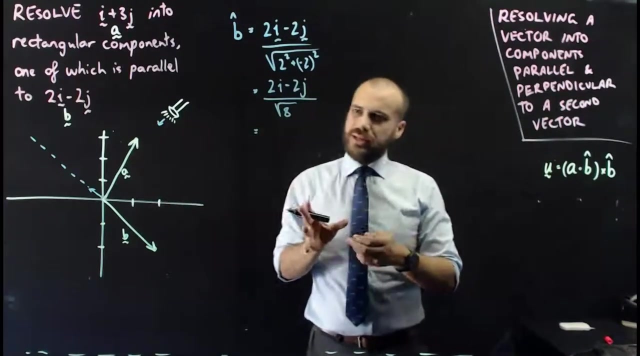 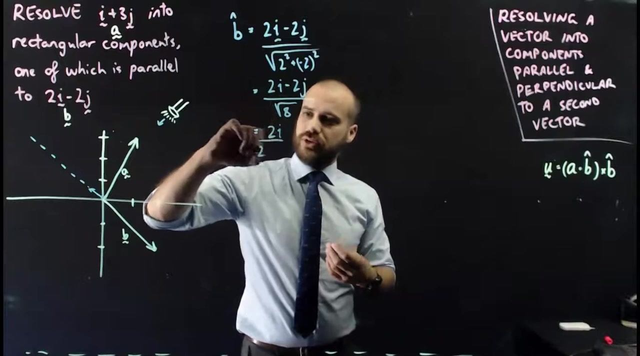 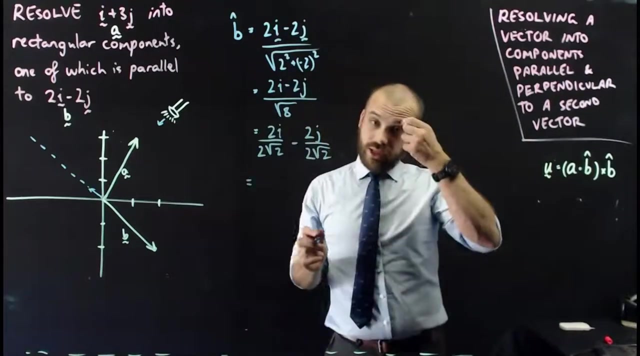 over the magnitude of vector b. so that's 2 squared plus negative 2 squared. all right, so that's going to be like 2i minus 2j over root 8, which can be made a little bit neater. root 8 is the same as 2 root 2, so now I've got 2i over 2 root 2 minus 2j over 2 root 2. that gives me a. 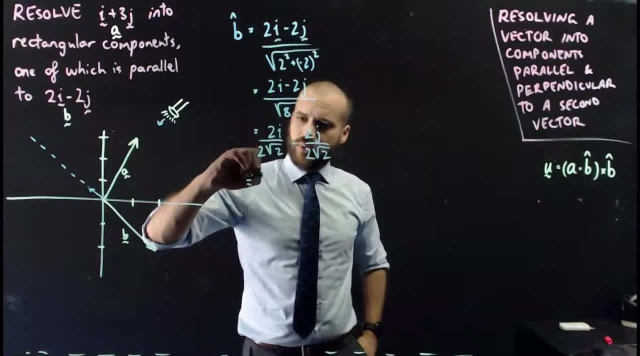 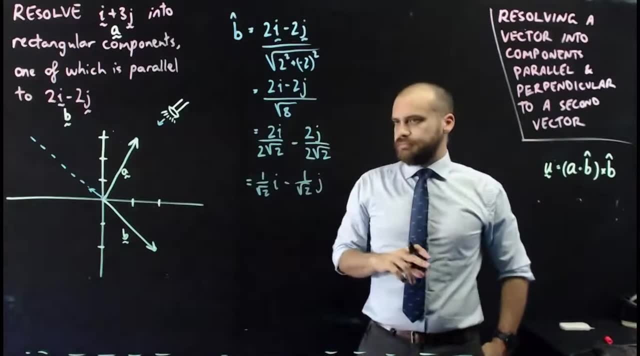 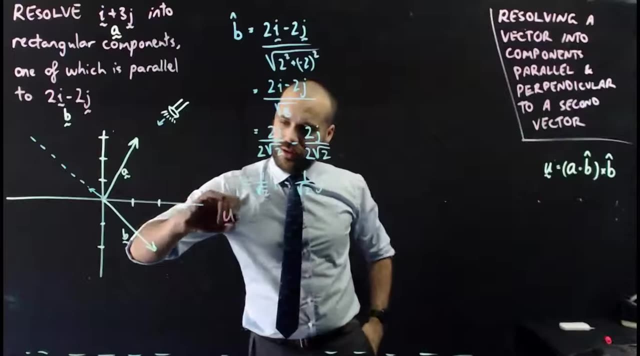 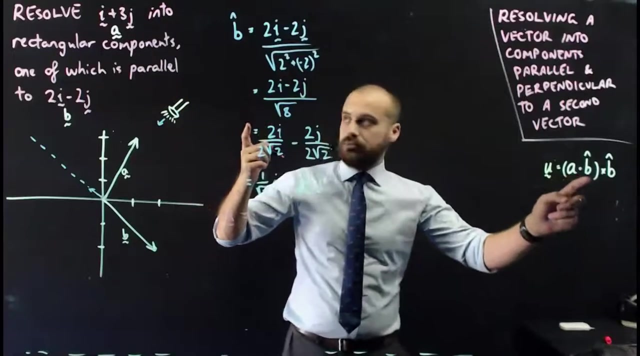 pretty neat little thing here: 1 over root 2i minus 1 over root 2j. so now that I have that I can do my whole vector projection here. so u is going to be the dot product of a now or a dot unit, vector b, so it's going to be 1 times. 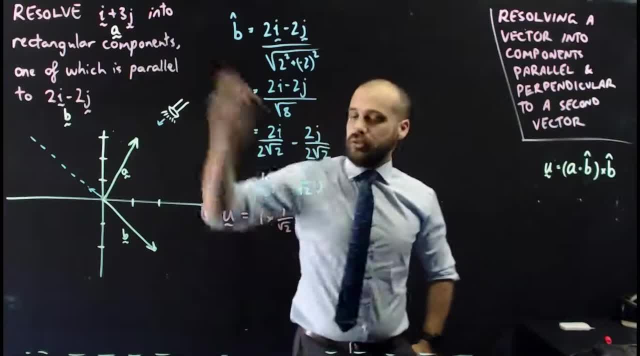 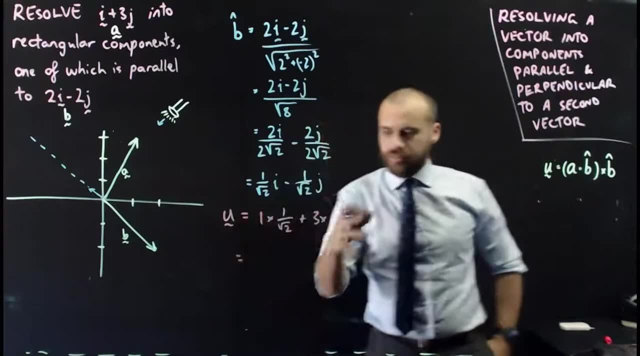 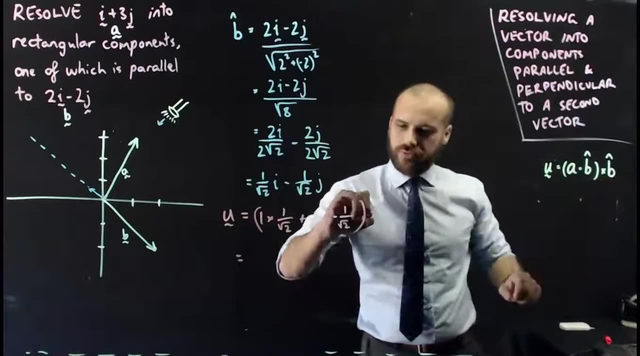 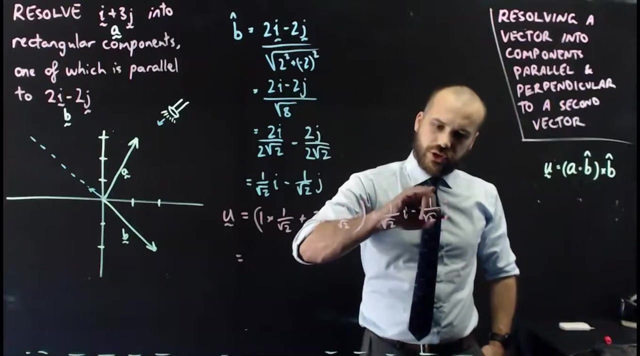 1 on root 2 plus 3 times negative 1 on root 2, and then I can calculate that. so I may as well keep going here. I'm doing the vector itself, so I need to multiply it by the unit vector then, and the unit vector is 1 on root 2i minus 1 on root 2j. now I'm going to take that and 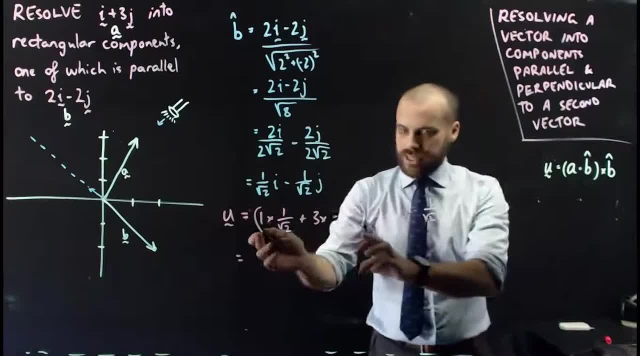 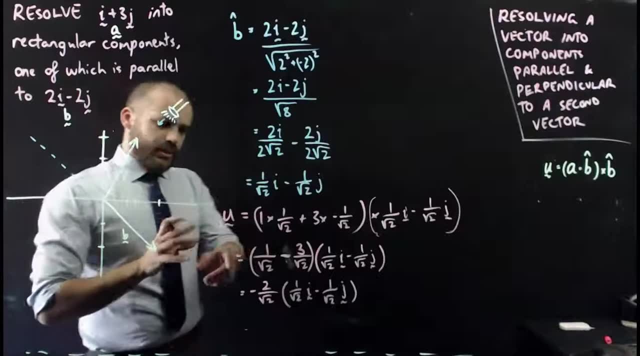 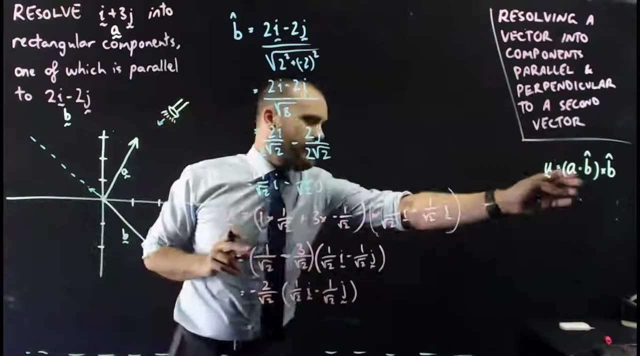 multiply that by that, that's going to be a single number. I'm going to take that single number, that scalar, and multiply it by our unit vector. try to skip ahead for you a little bit here. so I've just found out that our dot product of a dot unit vector b is going to be a dot product of a dot unit vector b. 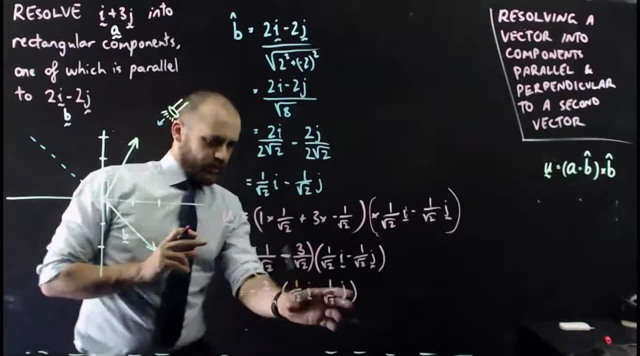 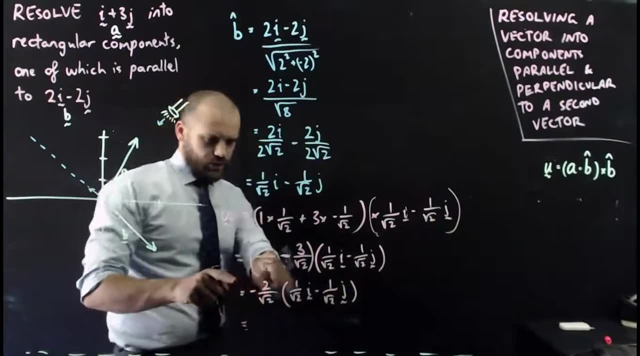 is negative 2 on root 2 and we're going to multiply that now by our unit vector b. now negative 2 over root 2 times 1 over root 2, that's going to be the same as negative 2 over 2, which is negative 1. so 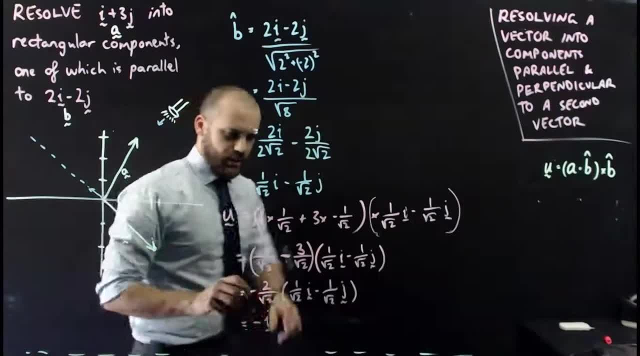 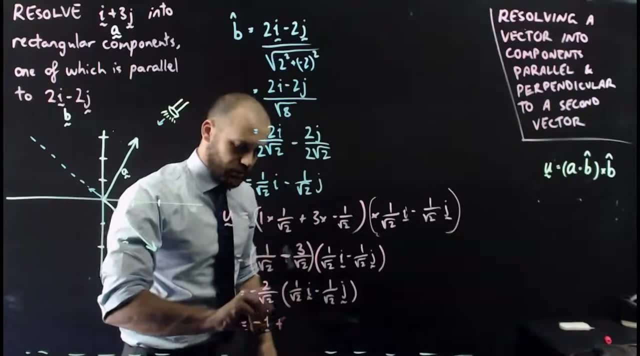 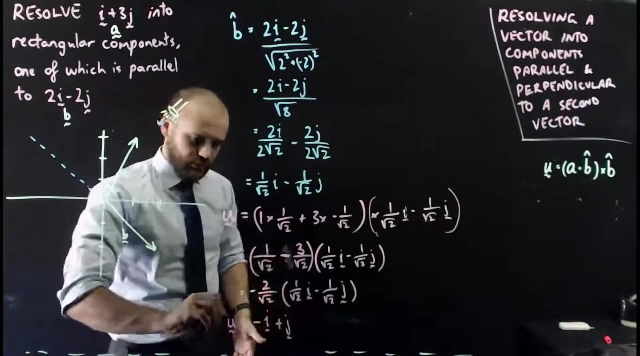 we just end up with a nice neat little negative i there and then negative 2 on root 2, times negative 1 on root 2. that's going to be positive 1. so now we end up with positive. j okay, now what? what is that? what is that thing? that's the shadow, that's, this is the 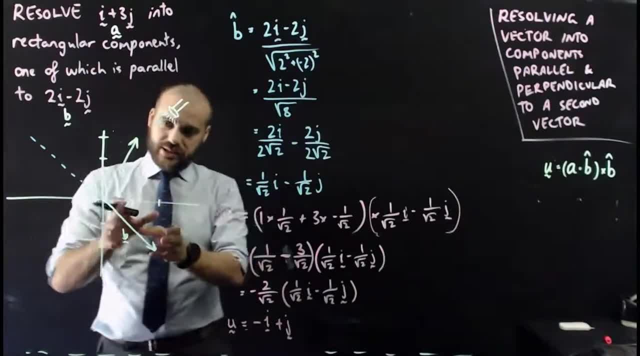 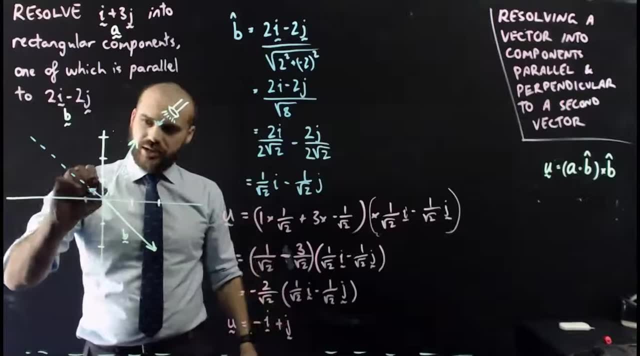 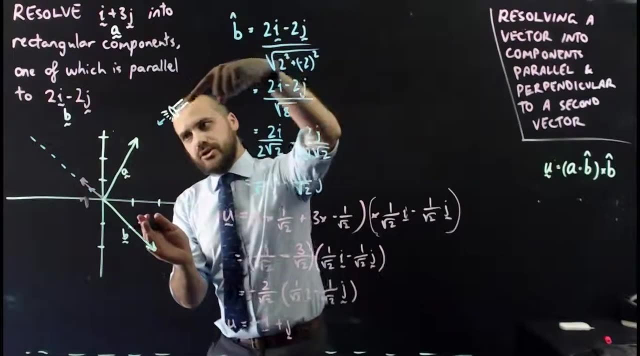 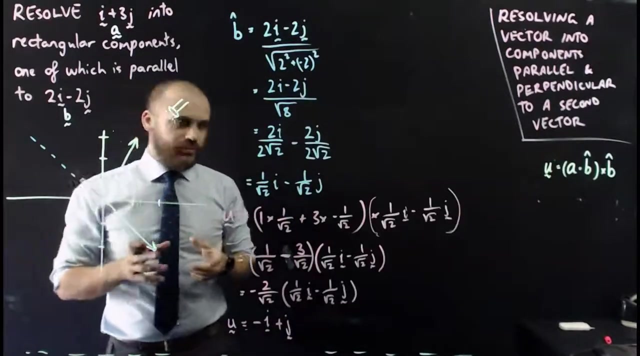 shadow that this vector is casting upon vector b, negative i here, positive j. okay, and you can see, here's my torch, here's my vector, there's the shadow. you know, obviously things aren't quite to scale, but you get the idea. now I'm halfway there because I'm supposed to. 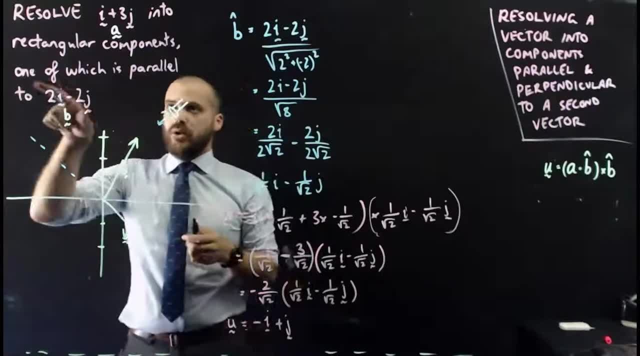 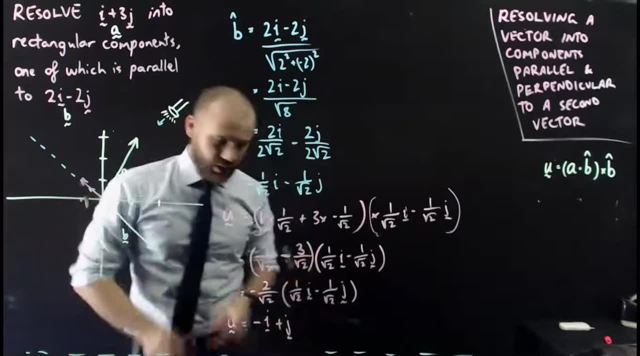 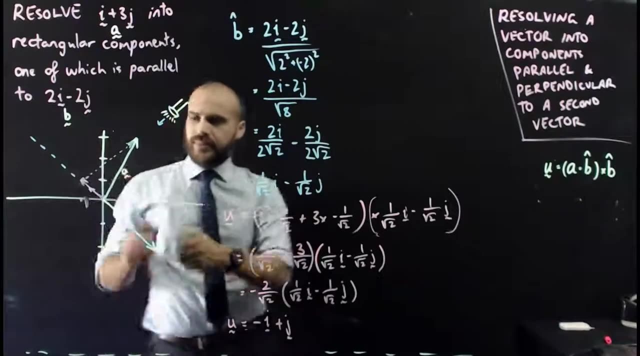 resolve i and 3j into rectangular components, one of which is parallel to 2i minus 2j. so I found the one that's parallel. the other thing I have to do now is find this vector here. so I know that vector, I know that vector. I need to find the blue vector. 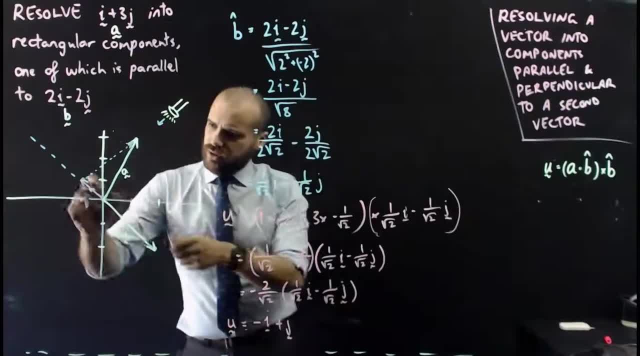 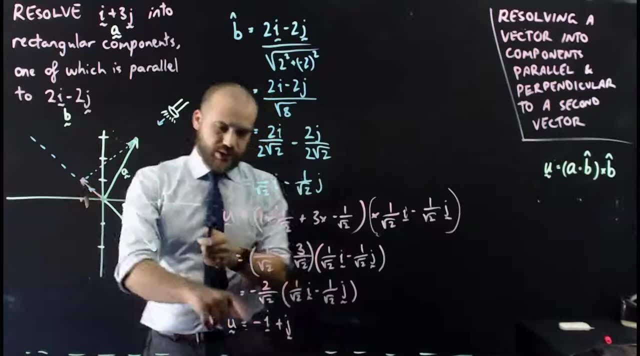 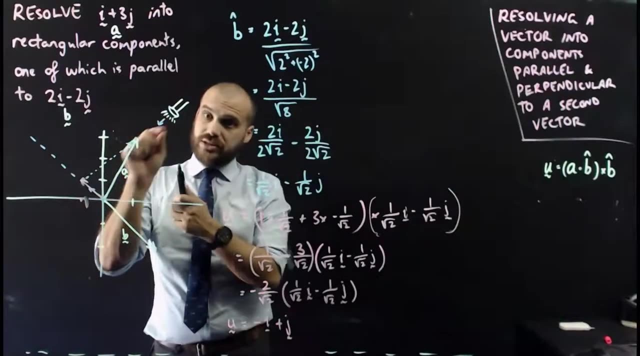 now, thankfully, if you look, we've got vector a is going from the point to the tip here and we found that vector. now, that pink one, it's negative y plus 2j, so we need to find that one. and it's always the case that when we're resolving vectors into rectangular components, if we add those rectangular, 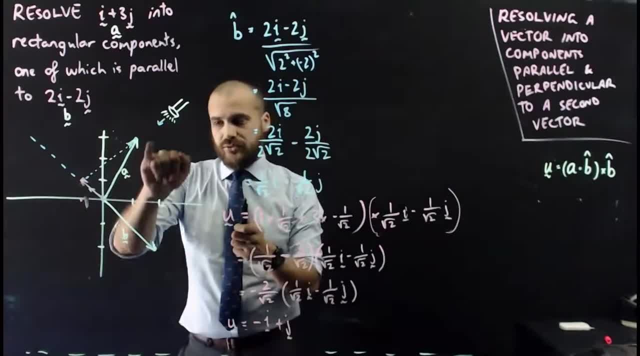 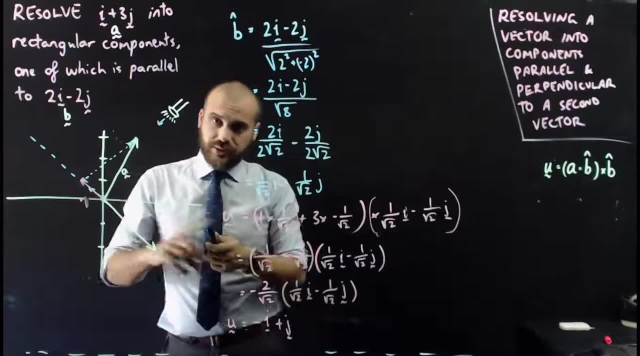 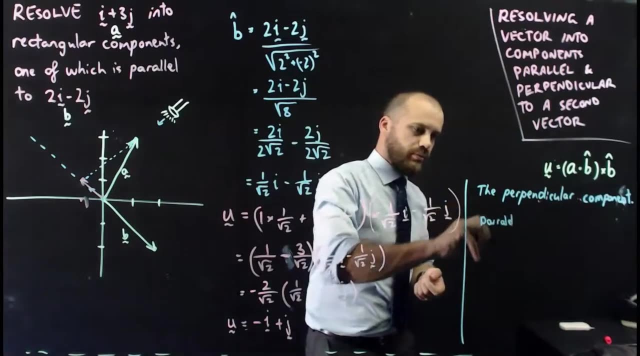 components together, we're obviously going to get that new vector which is adding them geometrically. we can also do like some subtraction to do that as well. so we're going to find that one and we're just going to repeat the process. so if what i'm going to call the parallel component 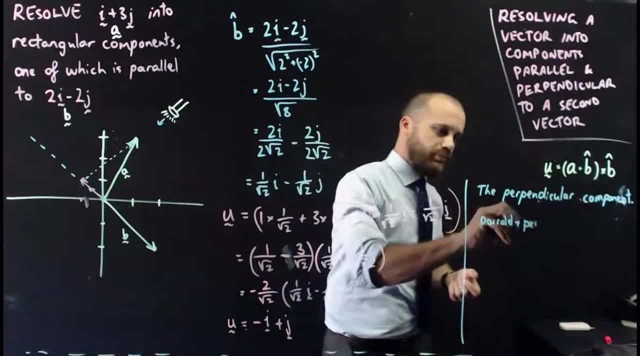 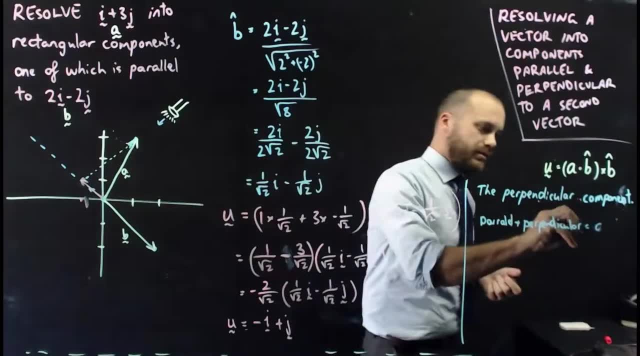 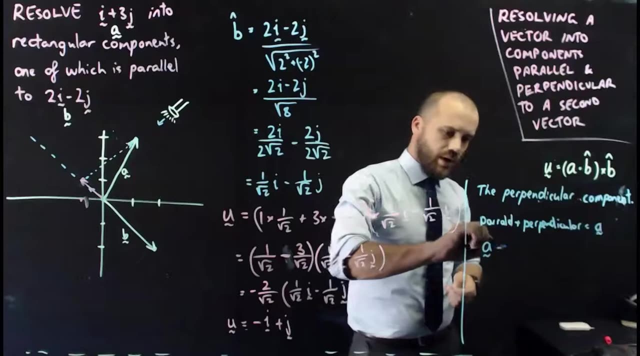 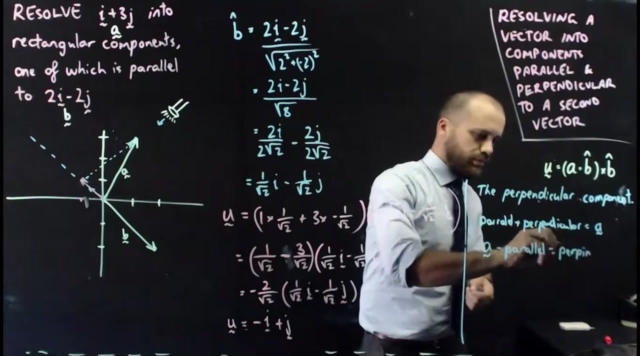 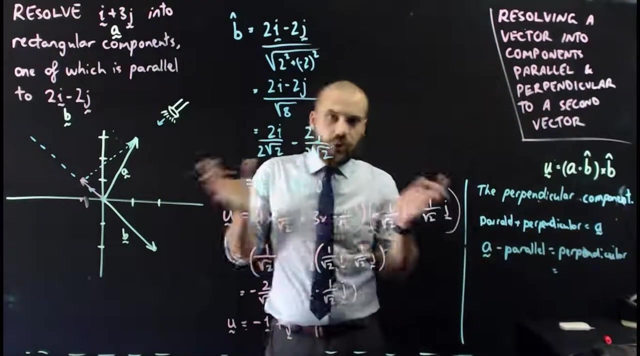 plus the blue one, which I could call the perpendicular component, equals that component, a. I can rearrange that right, so I can just say now that a minus the parallel component equals the perpendicular component. we've got to get that one and the perpendicular component, if I can spell, and that's. that's all we have to do for. 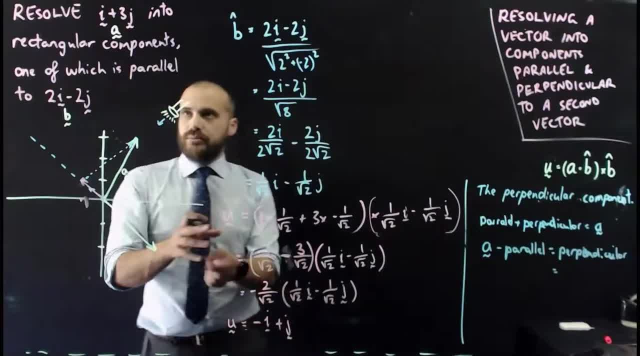 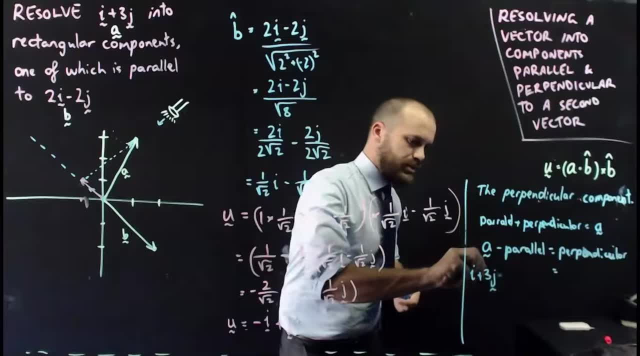 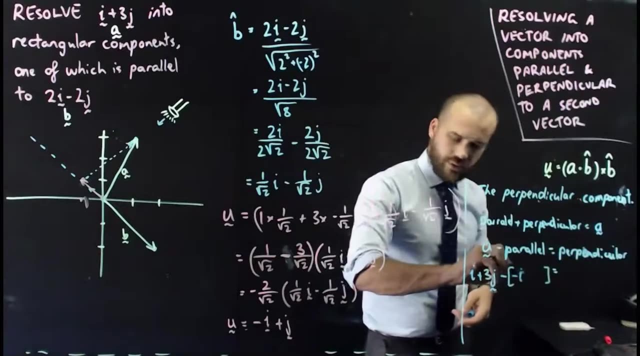 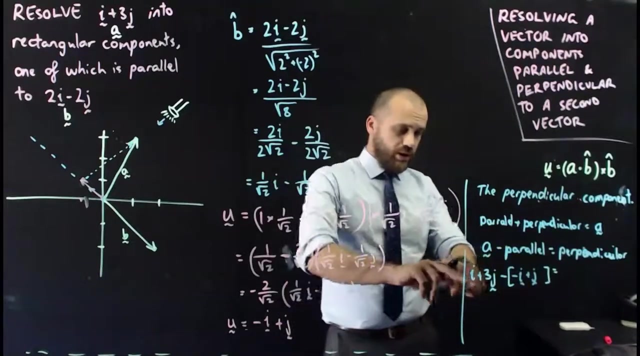 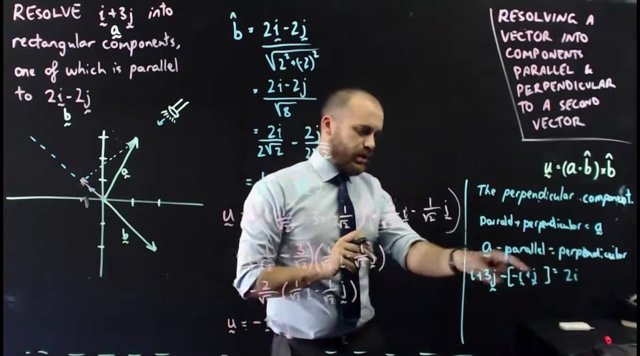 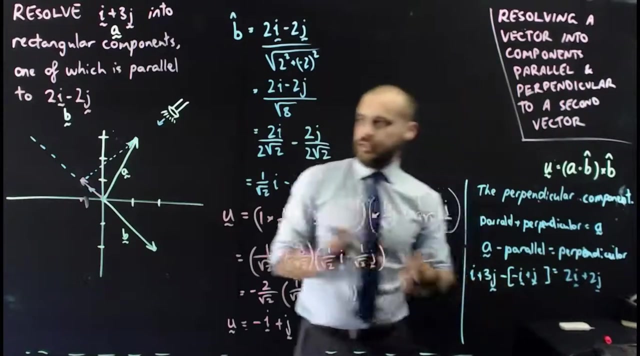 this last step, the vector projection, is kind of the hard bit. from here we just say, okay, well, vector a is i plus 3j. I need to subtract the vector that I resolved plus j, and now I'll know the perpendicular vector. so I minus minus I, it's 2i, and 3j minus j is 2j, and let's see if that kind of washes with. 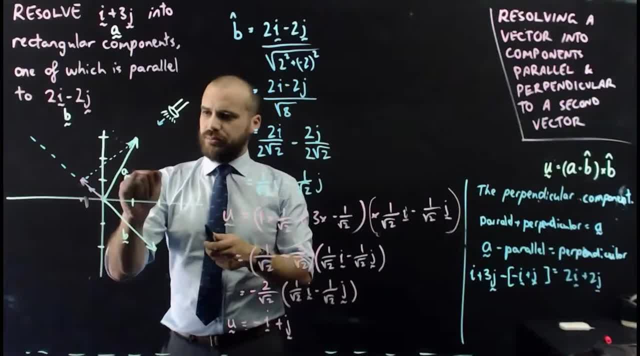 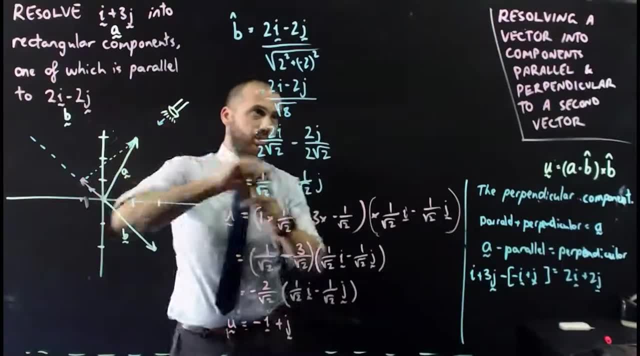 what we're doing. we're moving two across from that point to that point. we're moving two across from that point to that point. we're moving two across from that point to that point. we're moving 2 up from that point to that point. That makes sense. What's the final answer to that question? 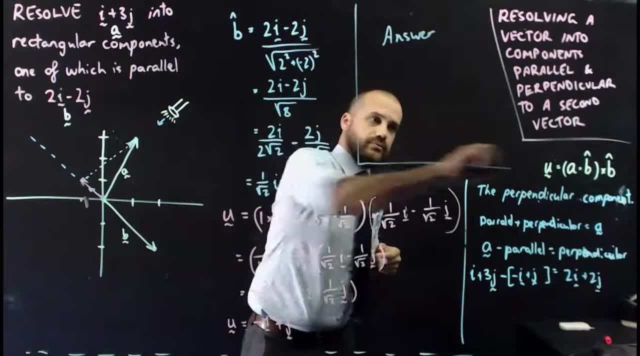 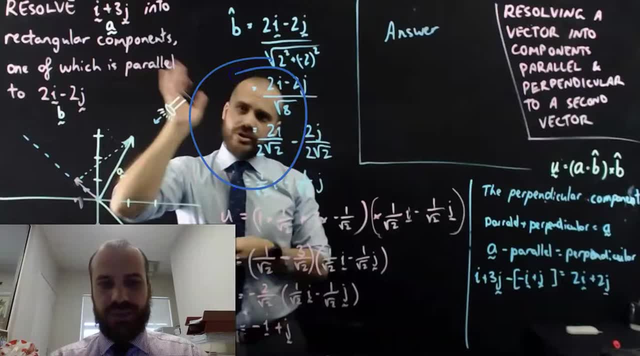 Answer: When I resolve, i plus 3j. All right, so I'm going to jump in here real quick because this guy here is going to make a bit of a mistake. All right, so let me show you what's really going on. 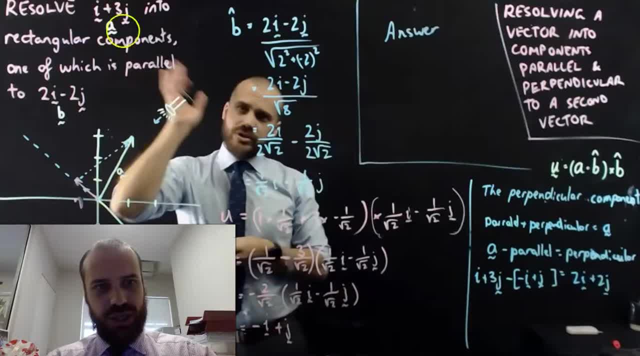 here. We've got this vector that we started with i plus 3j. We're resolving it into its rectangular components. Now one of them is this one here and the other one is this one here. So our final answer up here is going to look like this: Now, i plus 3j. i plus 3j is the thing we were trying. 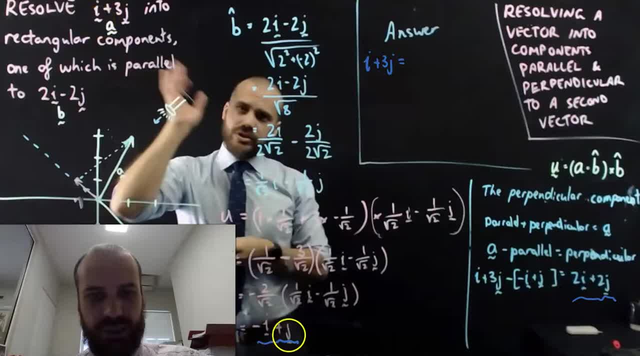 to resolve into rectangular components, and that's going to be equal to this one down here, which is i plus j plus this one down here. Now, it's not necessary, but I'm going to put my little brackets around here just to show that this is one vector and this is another one. Now, remember, 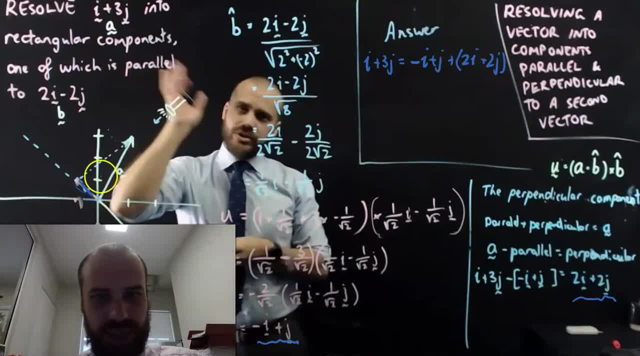 this vector is this vector right there and this vector is this vector right there. and combined they make this vector right there. That is, resolving a vector into components that are parallel and perpendicular to a second vector.